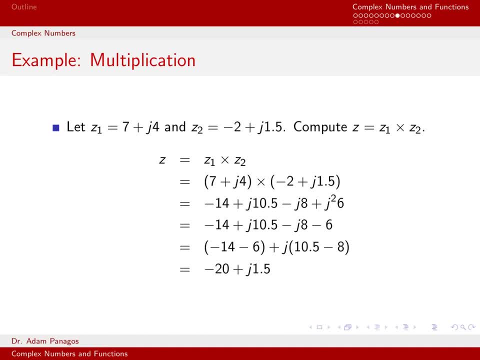 So that squared gives me n minus sign, so that turns into a negative 6.. And now I just combine like terms: I grab the real components which are negative 14 and negative 6, and I put those here. And I take the imaginary components which are 10.5 and 8, and I put those here. So a negative. 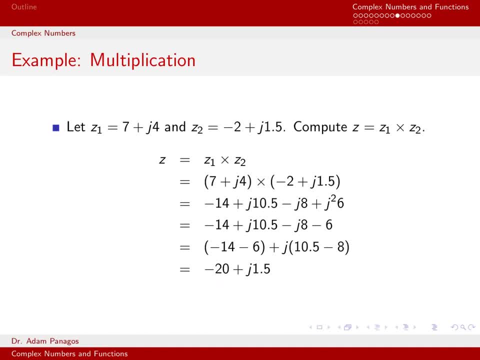 14 minus 6 is a negative 20.. And 10.5 minus 8 is 1.5, so I end up with j1.5.. Let's do an example of conjugation. This is almost trivial, but let's just do an example, to be. 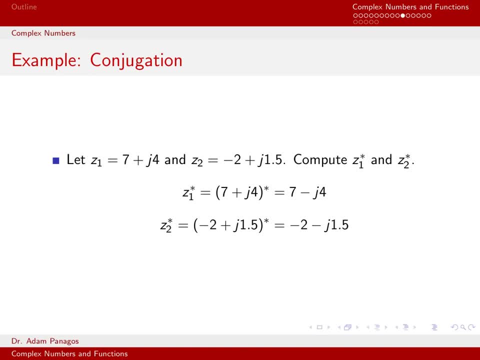 complete here Same numbers- z1 and z2, and I'm going to compute their conjugates: z1 conjugate and z2 conjugate. So, starting with z1, I write down what z1 is. I need to take the conjugate. 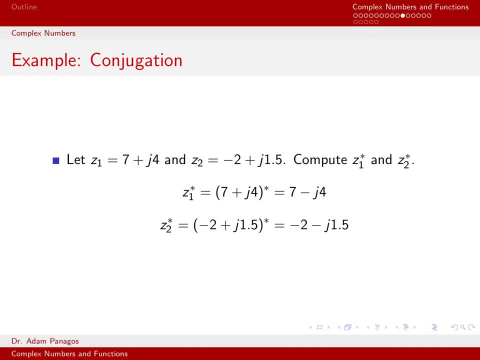 of this quantity. Remember what the conjugate does. It takes all the j's and turns them into negative j's. So this j right here gets replaced with a negative j, so we get the complex number 7 minus j4.. Similarly for z2, if I want to compute its conjugate, I write down z2.. I take the conjugate. 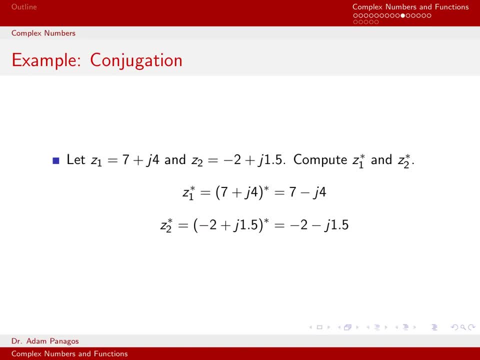 of the whole thing. and then everywhere in here where I see a j, I change it to a negative j, so I end up with a negative 2 minus j times 1.5.. So we've computed the conjugate of z1. 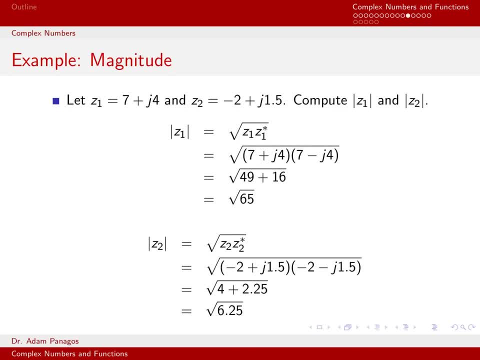 and the conjugate of z2.. Next let's do an example of computing the magnitude of some complex numbers. So the same z1 and z2 we've been working with, and now I'm going to compute the magnitude of z1 and the magnitude of z2.. 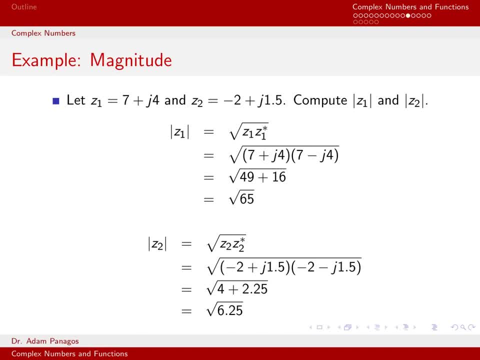 So to compute the magnitude of z1, remember, by definition, the magnitude of a complex number is the square root of the complex number times its complex conjugate. So we know what z1 is. so I put it right here. We just computed what the conjugate of z1 is: It's z minus. 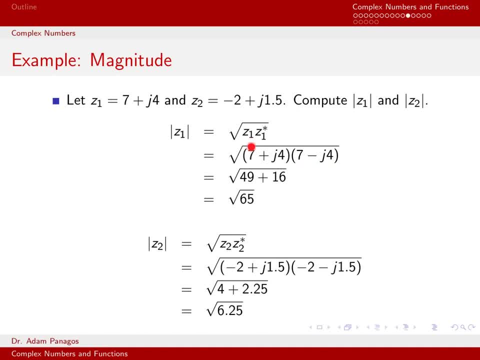 j4. To compute this product, we know how to do that. It's just the first. so 7 times 7 is 49, then plus the outer, which is 7 times a negative j4, plus the inner, which is j4. 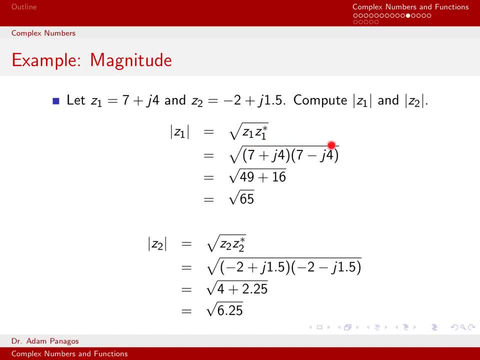 times 7, so those cancel. This term gives me a negative 28j. this term gives me plus 28j, so those are going to cancel. And then the last term is going to multiply and give me a j squared which is negative. 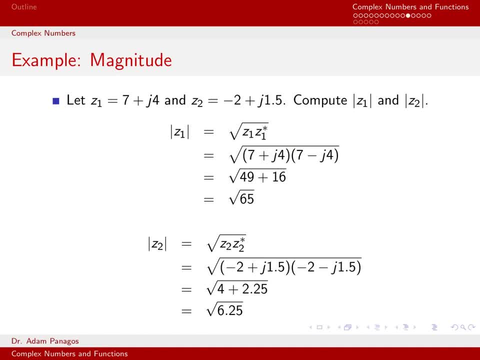 so it cancels this negative, turns it positive, and 4 times 4 is 16.. So this always happens when we compute the magnitude. These inner terms always cancel and you're really just left with this squared plus this squared, So 49 plus 16, if you add that together, you 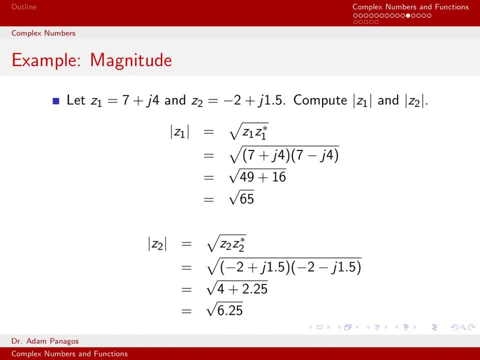 get 65.. So the magnitude of z1 is the square root of z2, plus the inner, which is 6 times the square root of 65.. We can do the exact same steps to compute the magnitude of z2.. By definition, the magnitude 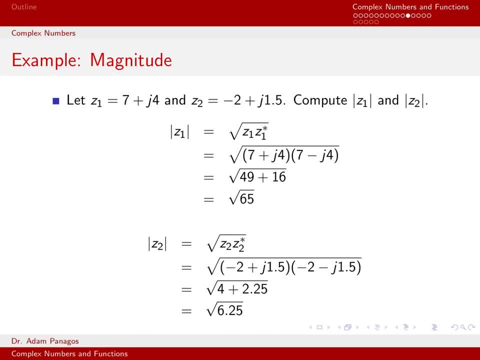 of a complex number is the square root of itself, times its complex conjugate. so that's what I have right here. If we want to think about this how we did before, what I end up with here, after the things cancel are just this first term squared, so a negative 2 squared is 4, and there's 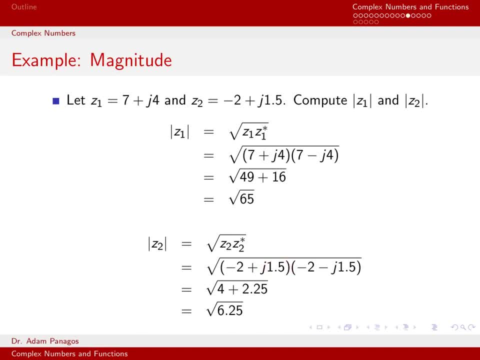 a last term: squared 1.5 squared is 2.25.. So if I add those two together, 4 plus 2.25 is 6.25.. So the magnitude of z2 is the square root of 6.25.. 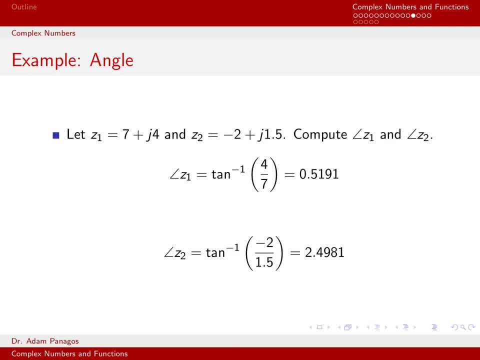 Let's go ahead and do the angle computation Now. we just computed their magnitude. Let's compute their angle or phase as well. So if I want to compute the angle of z1, remember how we do that. We take the tan inverse of the imaginary component divided by the real. 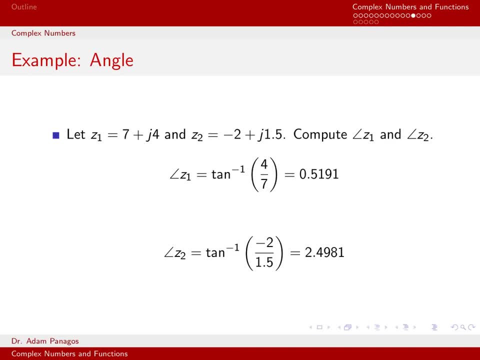 component. So the imaginary component of z1 is 4, and the real component of z1 is 6.. So if I plug this into my calculator, the tan inverse of 4 sevenths is 0.5191, and this is in radians. This is not degrees. Similarly, to compute the angle of z2, I take the tan. 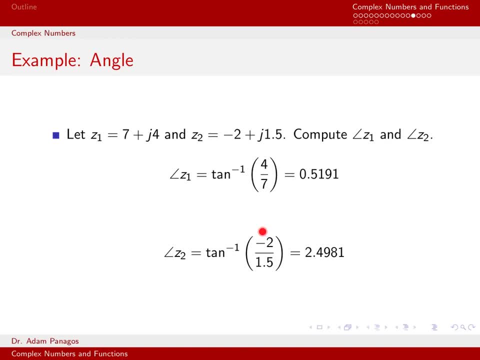 inverse of the real part, which is a negative 2, so that goes in the numerator divided by the imaginary part of z2.. If I look at z2, the imaginary part is 1.5, so that goes onto the denominator Again. if I use my calculator to compute this quantity, I get 2.5 squared. 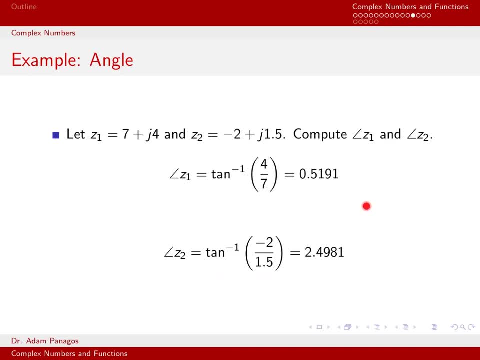 So that's 2.4981 radians. So we now know what the phase or angle of these complex numbers is. Let's go ahead and write these complex numbers in polar format. now Remember what polar format is. It's a way to write a complex number in terms of its magnitude, times e raised to its 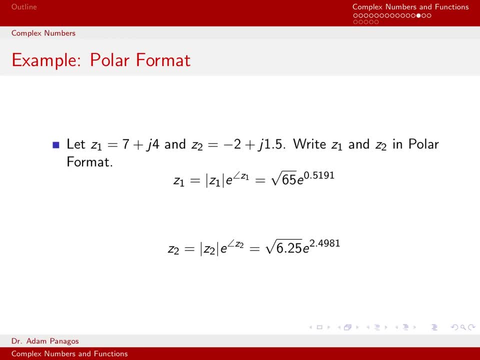 phase. So we've already done these computations. We computed the magnitude of z1.. We found that it was equal to the square root of 65.. And on the very last slide, we computed the angle of z1 and found that it was equal to 2.4981 radians. So we've already done these. 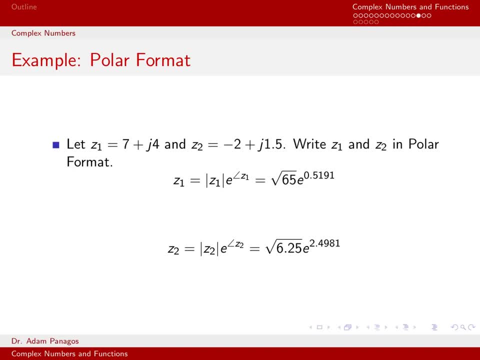 computations. So we know that z1 is in the rectangular form of z1 plus j4.. And the equivalent way to write z1 is in polar format. so it's square root of 65 times e to the point 5191.. Same thing for z2.. z2 in polar format is the magnitude of z2 e raised to the angle of z2.. 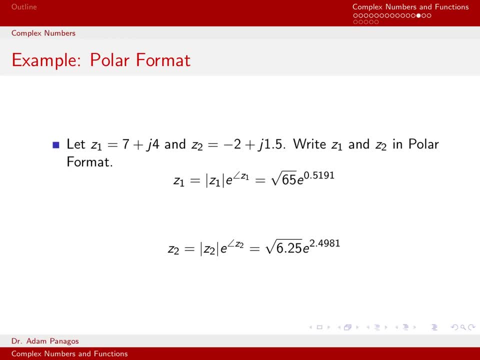 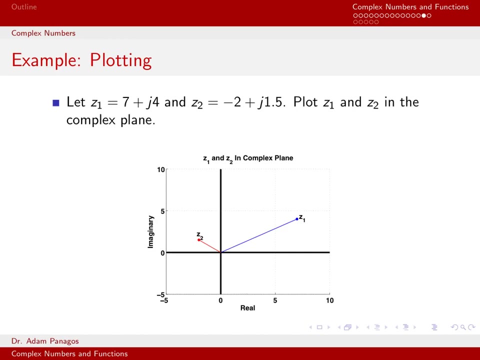 Well, we just did these computations. so that's square root of 6.25 times e to the 2.4991. Let's go ahead and plot these complex numbers in the complex plane now. So here is a plot of the numbers z1 and z2, and I can think of this any way that I want. 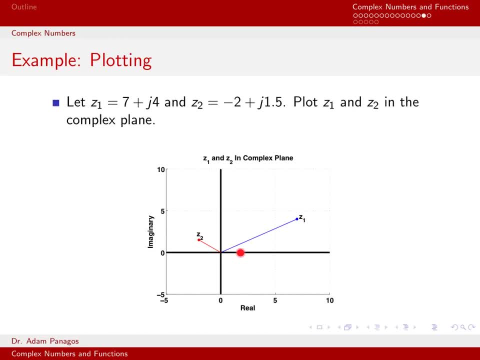 I can think of it in rectangular form. I can think of z1 as coming out 7 and then going up 4 and landing right there on that dot z1, right here. Or I can think about it as going out a magnitude- what was it? square root of 65, and then rotating. 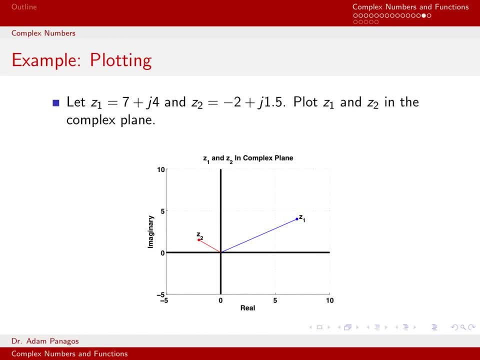 up about 0.5 radians and I would end up in that exact same spot. Same thing for z2.. One way to think about plotting z2 is to come on the real axis, down negative 2, and then going up on the imaginary axis 1.5 to end at this spot, right here. 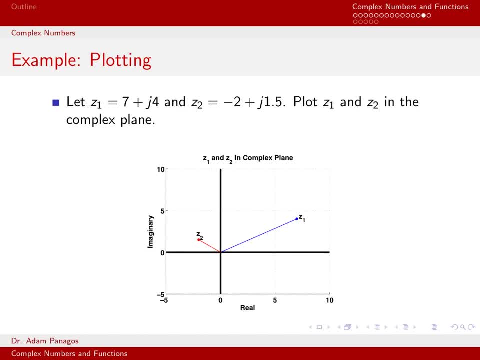 The other way to think about it is to come out on the real axis- square root of 6.25, and then rotate about 2.5 radians and end up right there at that spot. So no matter whether you think about it or not, you can think of it as coming out of. 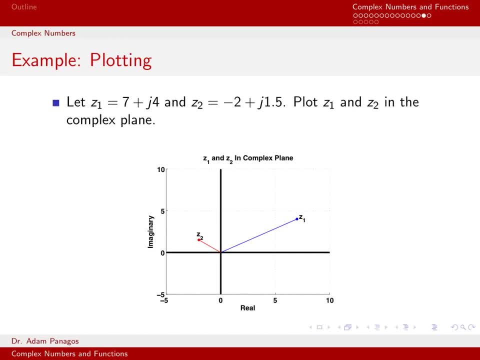 0.5 radians. You can think of it in terms of rectangular coordinates or in terms of polar coordinates, like we just did on the previous slide. Those are both identical. They give you the exact same spot on the complex plane. It just depends on how you want to think about it. 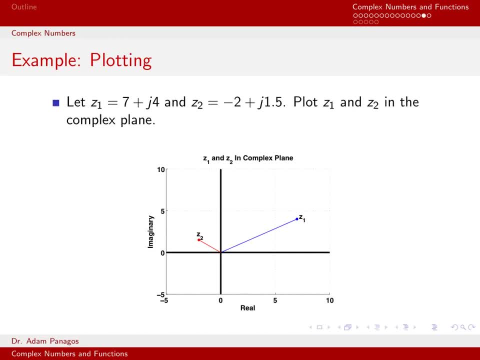 So that concludes this video of working some very specific examples of performing operations on complex numbers. We did addition, We did multiplication, conjugation, computing the magnitude, computing the angle and plotting complex numbers in the complex plane. Thank you, And the next video we'll actually walk through doing these operations in MATLAB.